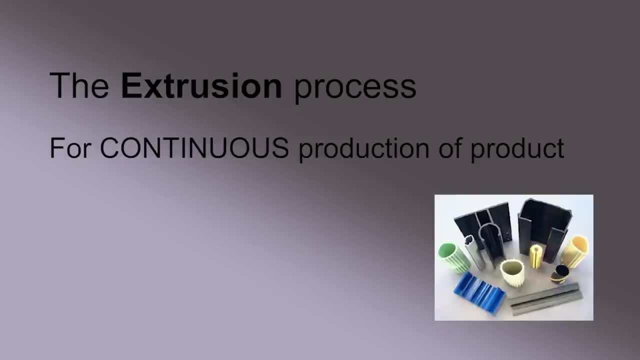 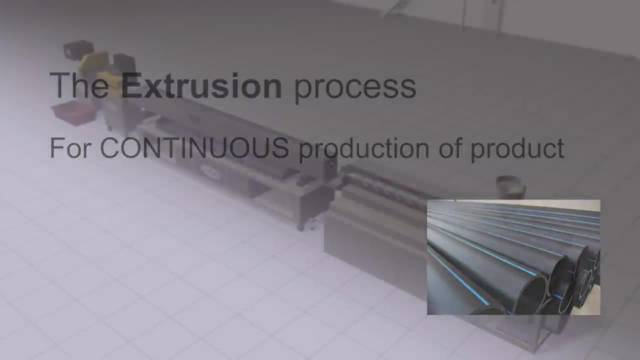 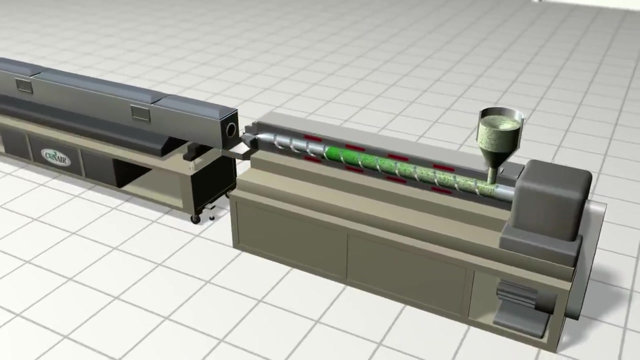 operation as injection molding, but there is no mold and the resin compressing screw rotates constantly and product is created continuously. Extrusion uses a die, a hollow form that molten plastic is pushed through to create its specific shape and thickness- A water bath or spray chamber. then cool the extruded. 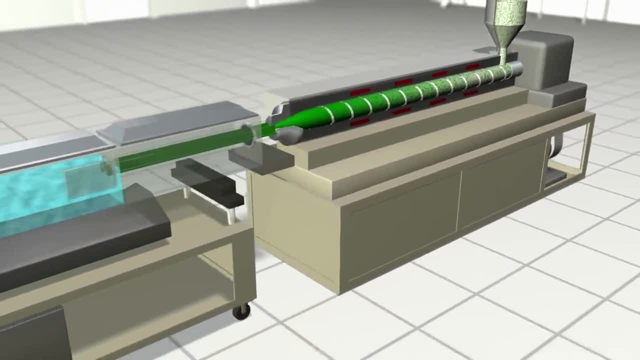 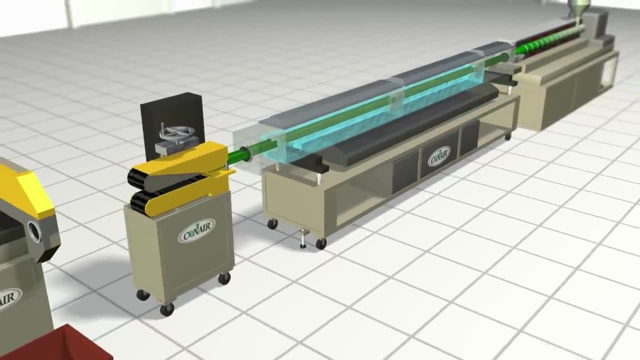 shape and often provide pressure and or vacuum controls to properly size the product as it passes through Belts or cleated. pullers apply smooth tension on the product and keep it moving in pace with the extruder. A cutter or saw create the final product length or a winder. 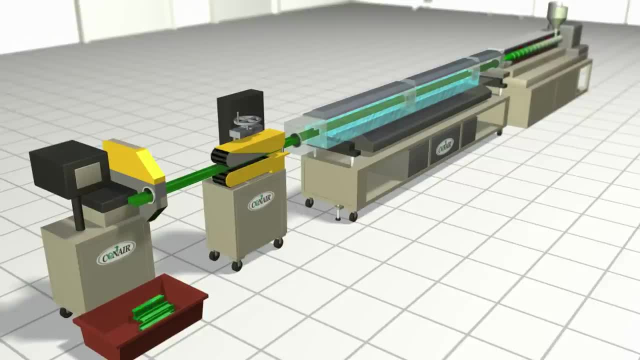 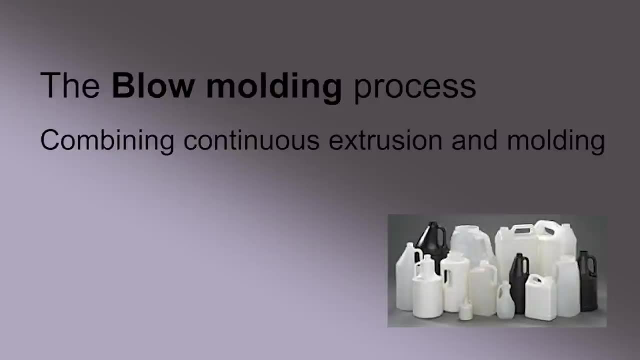 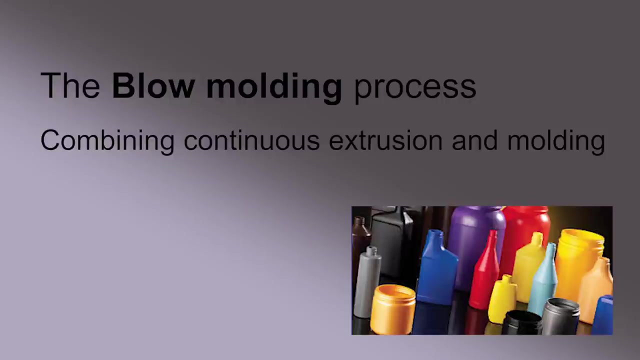 creates spools of the final product. There are many variations to the extrusion process, but a mixture of extrusion and molding is found in the blow molding process. plastic is continuously extruded into a tube shape and then clamped in a mold and blown into its shape with compressed air. It's a process that often operates. 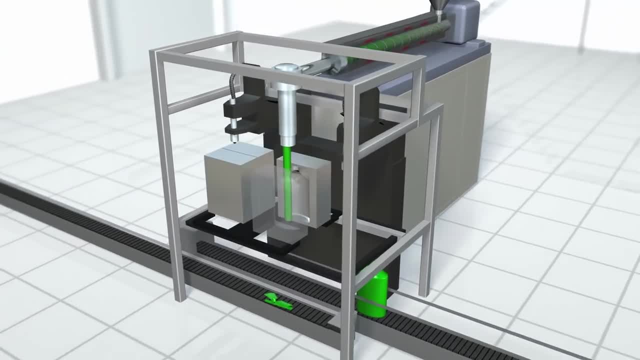 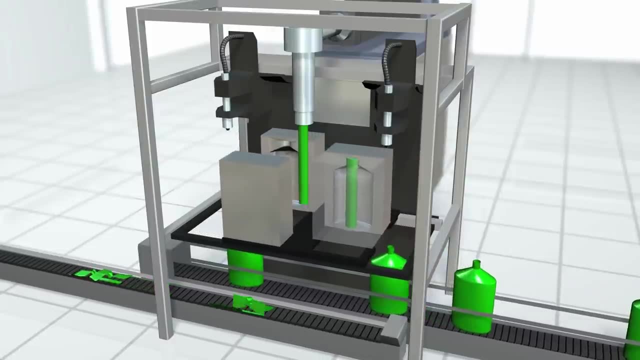 in a shuttle movement with a set of molds. Each mold takes a turn, grabbing a section of extruded tube called a parison and shuttling it to one side to blow it into a bottle shape, letting it cool and then releasing it to be filled. 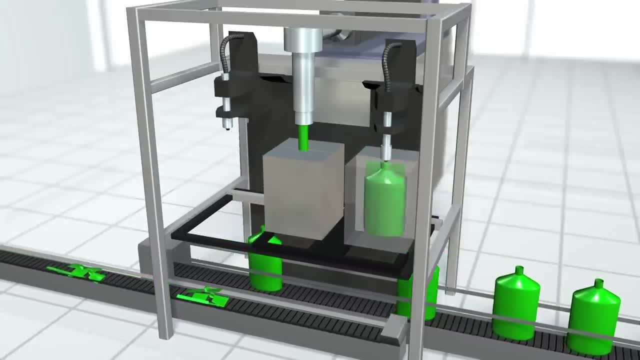 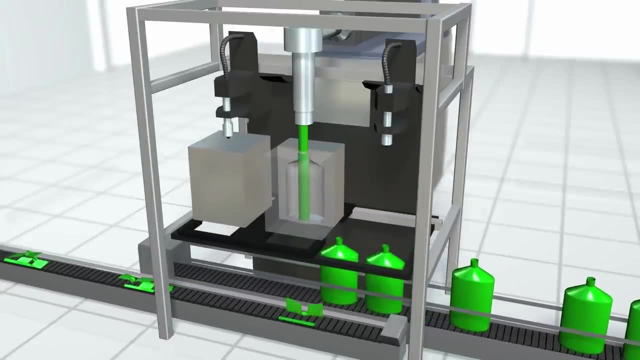 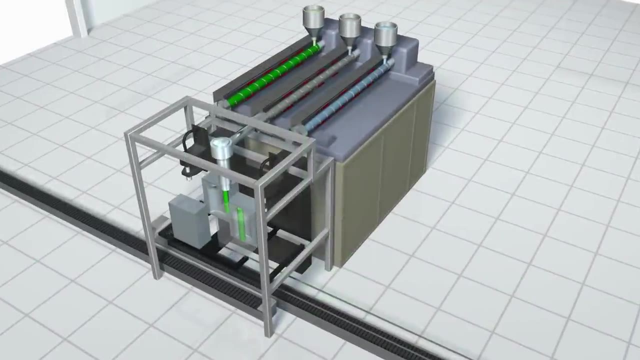 with product or shipped. Each mold alternates with a second mold doing the same thing for maximum productivity. The same blow molding process can also utilize multiple extruders for what is called co-extrusion. Co-extrusion is used to create bottles made up of multiple 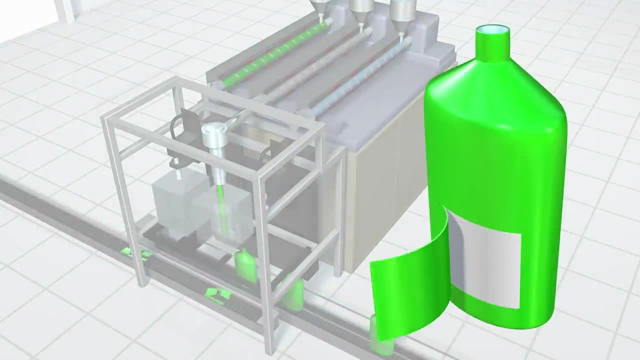 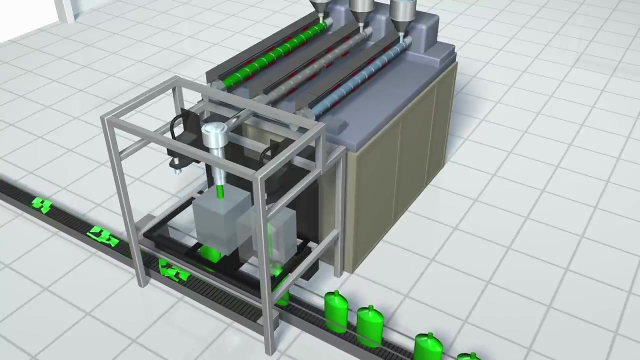 layers, and each layer possesses special characteristics like suitability for food contact, an outside color for brand awareness, ultraviolet light protection for long shelf life of the product, a layer of regrind for economical reuse of scrap, and many times, barrier and adhesive layers are included to separate and bond the layers for a tough, cohesive. 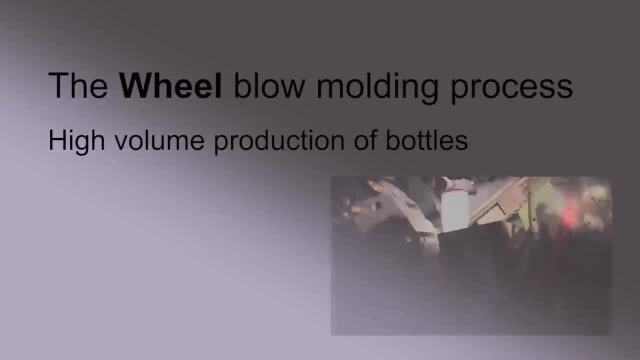 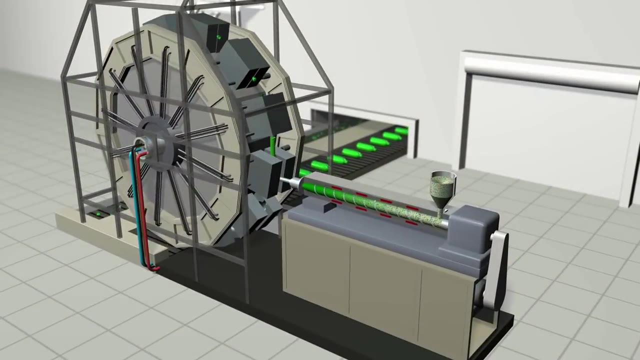 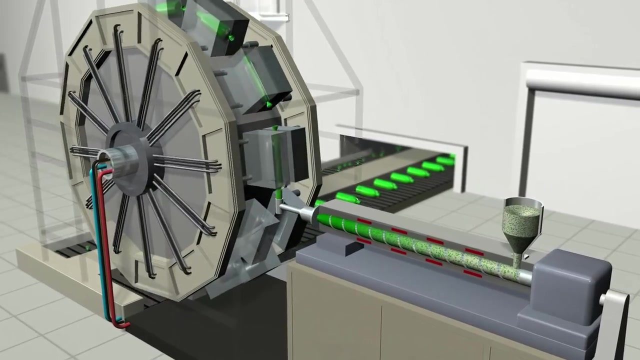 bottle. A high-volume form of blow molding uses many molds mounted onto a continuously rotating wheel mechanism. The extruder creates a hollow tube and as the wheel rotates, each of its molds will open. grab a parison from the extruder, die. blow the parison into a bottle.